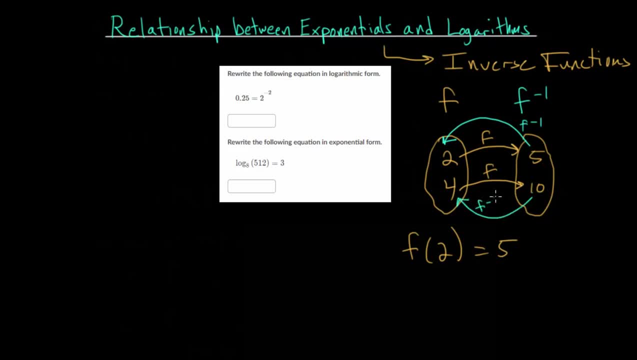 inverse function or the inverse mapping goes in the reverse direction. so we can say that the inverse of 5 is equal to 2 and, formally speaking, inverse functions. if we want a better definition, tell us that F of a. when we put a into our function, that specific value, it would, let's say, give us a value of B, the 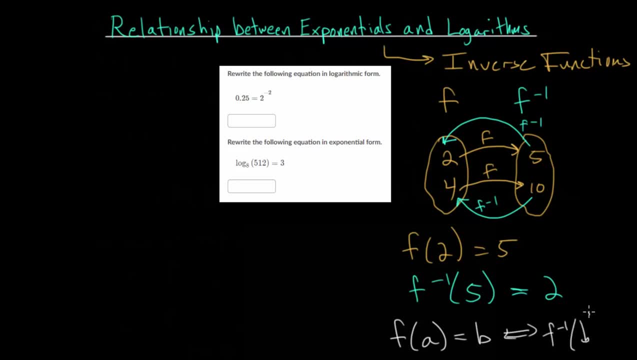 inverse to this. if we plug B into our function, it will give us an output of a. so inverse functions reverse each other, and exponential and logarithmic functions are inverse functions of each other. so let's look at a specific example before we jump into any of these problems here. 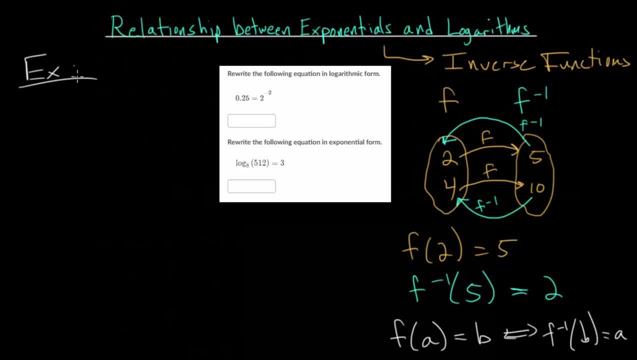 just so that we can understand the relationship a little bit better. let's say we have the exponential function y equals 10 to the axe and we want to find its inverse. so the first step when you're finding an inverse to, let's say we are going to invert this. 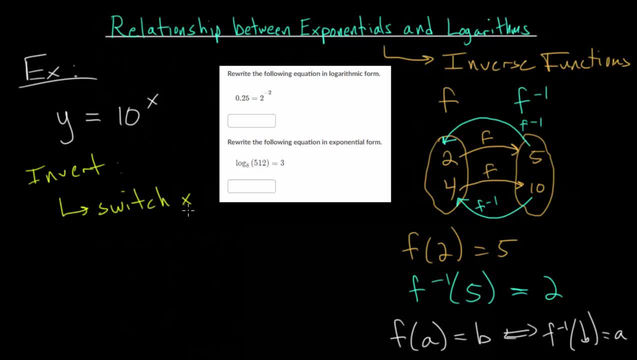 to switch the x and y values and by switching them we can find that inverse function. they switch because we're essentially reversing the function process and if you want, you can call this f of X. and so we're finding F inverse of X. and so to switch them, we get X equals 10 to the Y. and our next: 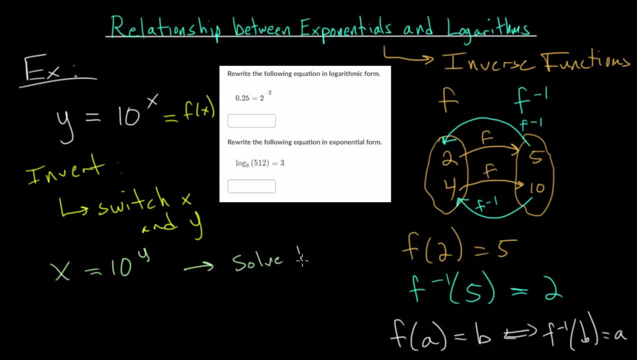 step to find that inverse function we need to solve for Y. so to do that, since Y is in the exponent, we can rewrite this as a logarithm. so remember that when you're rewriting a logarithm, so we'll have log with a base, the base of the. 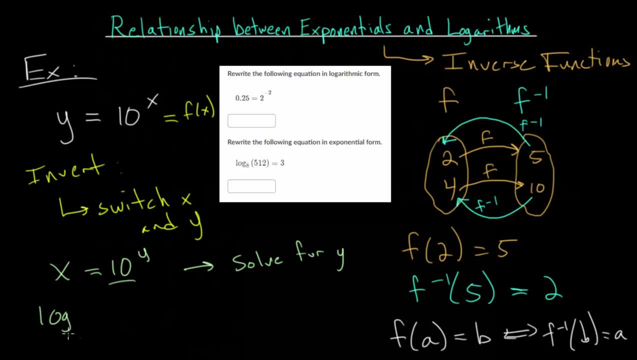 logarithm is always the base of your exponential expression. so this will be a log, base 10, which is the common log, and so eventually we don't even have to write the base tense: it's. if you see log, you can write it as a common log, and so eventually we don't even have to write the base tense: it's if you see log. 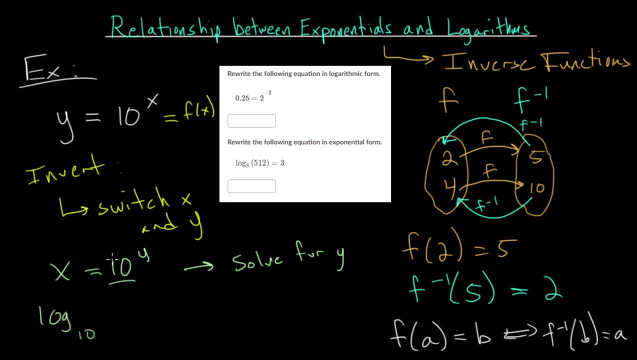 it's just assumed that the base is 10 and the logarithm is always equal to the exponent. logarithms are exponents and so process of elimination. the X would go on the inside of our logarithm, or you could remember that the input of the logarithm 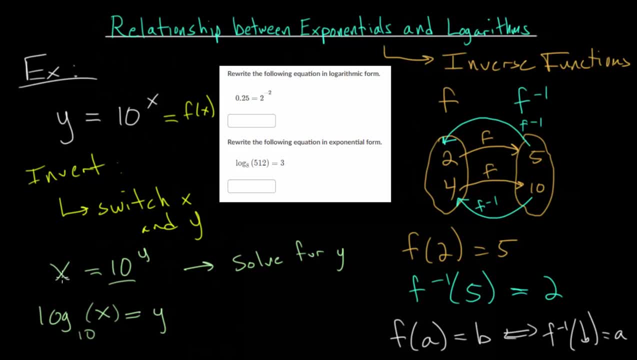 is always what the exponential expression is equal to. so we have this new equation: Y equals log, base 10 of X, which, like I mentioned, we can really just write as log X, since this is the common log and base 10 is bye hyder, which costed $10,000. so we end up with l. 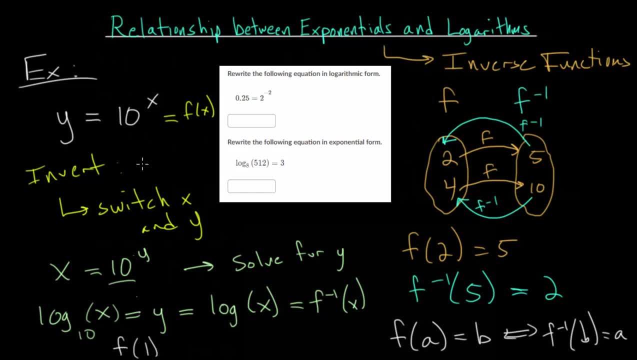 a million and now double check that this is true because, going by this definition, let's say we plug in the point into our original function of one, we'll plug in an X value of one, and that's just 10, 2, the first, which is 10, and so in our inverse function, be. 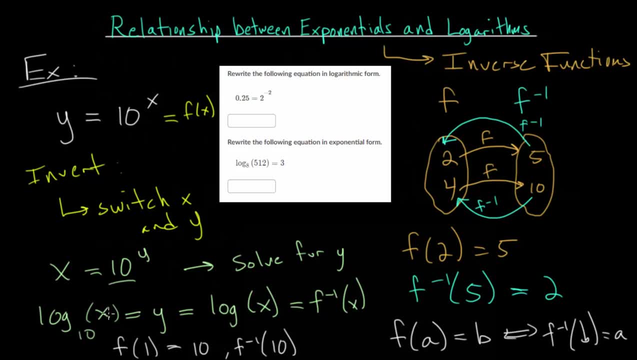 When we plug in 10, now we're doing log base 10 of 10.. So we ask: what power do we raise 10 to to get 10?? And we would raise 10 to the first power to equal 10.. 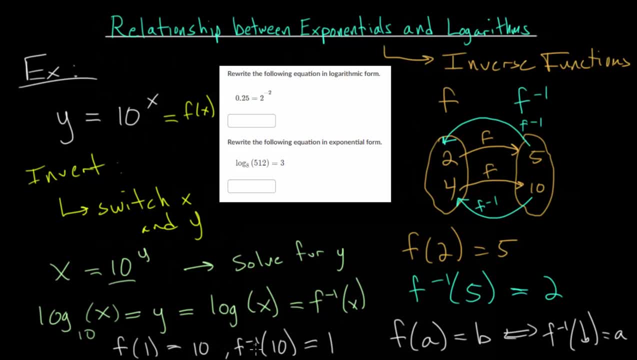 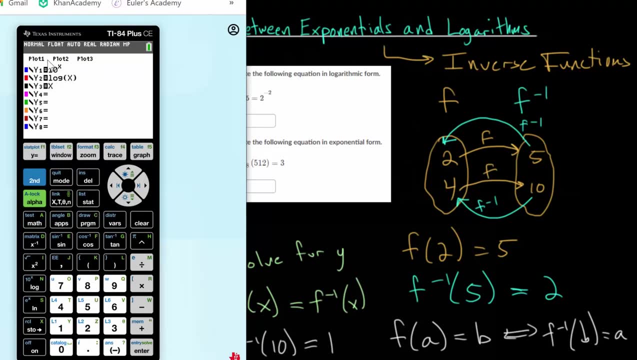 So you can see that the definition is satisfied. And just to further understand this, let's look at a picture of this. So let's get out the graphing calculator And I've already typed in our functions 10 to the x and log of x. 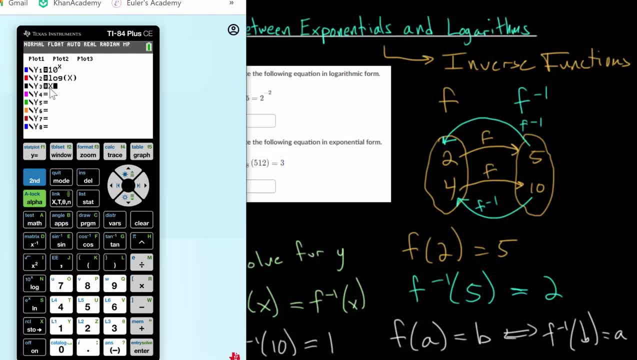 We do have a common log button here, And I've also put in the equation y equals x, Because with inverse functions, when we graph them they're always a mirror image about this line y equals x And you can see that symmetry here. 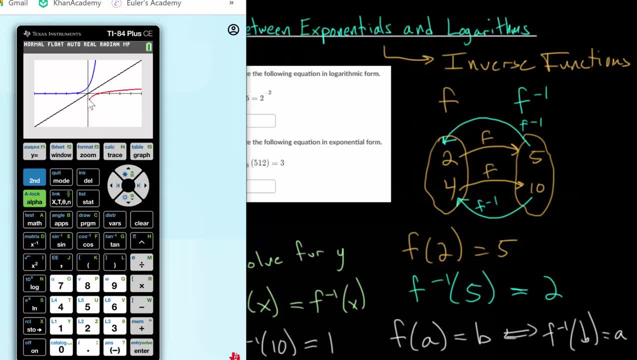 Now notice the red one's kind of cut off. That's just because it does not exist for x values less than zero or equal to zero. But if we were to zoom in here, we would see that this line actually just continues down and hugs this y-axis here. 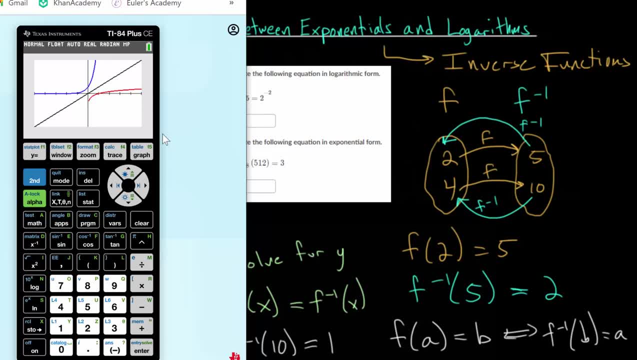 So if you look at these functions from a higher level- sort of a big picture- you can think that exponential functions grow incredibly fast And logarithmic functions, since they're the inverse, they grow incredibly slowly. But this nice symmetry does indicate that 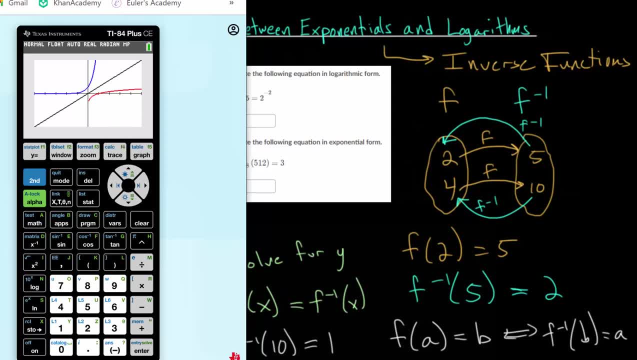 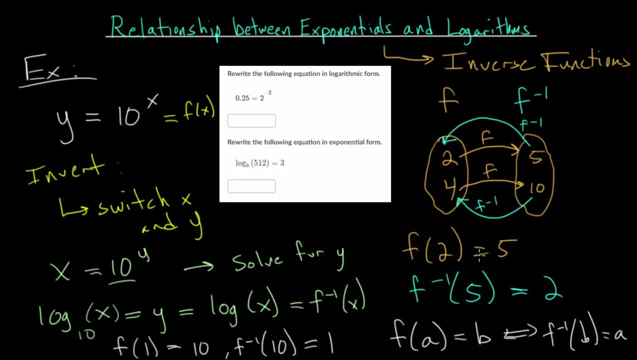 they're in fact inverses of each other. So with that in mind, let's start doing some of the example problems. I will clear some space and then we can go through the exercises. Here we go.